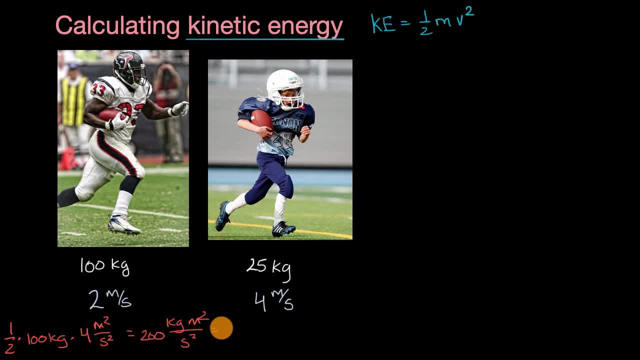 Or this is the unit of force times distance. And this is the unit of force times distance. This is the units of energy which we can write as 200 joules. Now let's do the same thing for this running back. that has less mass. 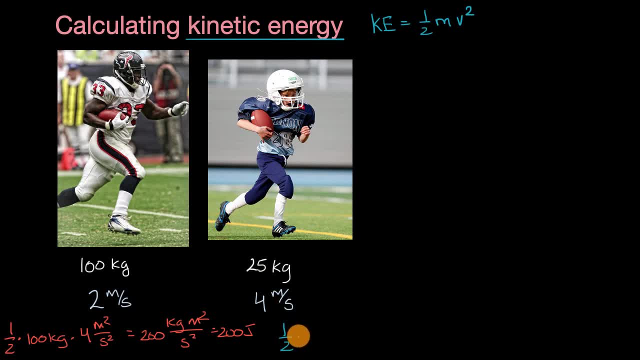 Kinetic energy here is going to be 1 half times the mass, 25 kilograms times the square of the speed here. so that's going to be 16 meters squared per second squared, And then that gets us. we're essentially going to have: 1 half times 16 is 8 times 25,, 200.. 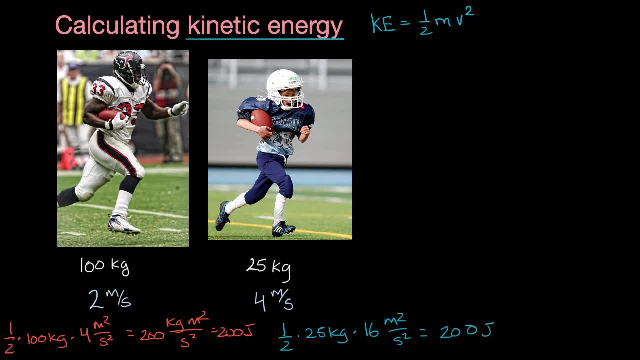 And we get the exact same units and so we can go straight to 200 joules. So it turns out that they have the exact same kinetic energy, Even though the gentleman on the right has 1 fourth the mass and only twice the speed. 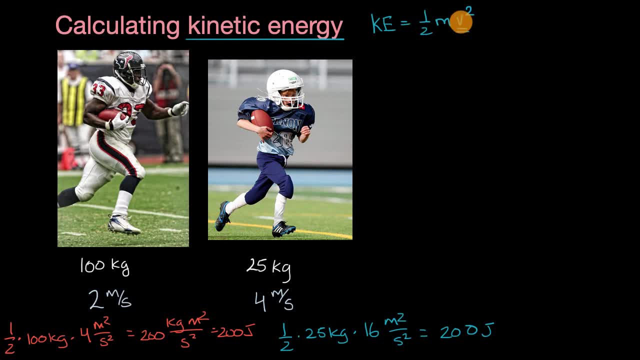 we see that we square the speed right over here, so that makes a huge difference. And so their energy. due to their motion, they have the same capacity to do work. Now some of you are thinking: where does this formula come from? And one way to think about work and energy. 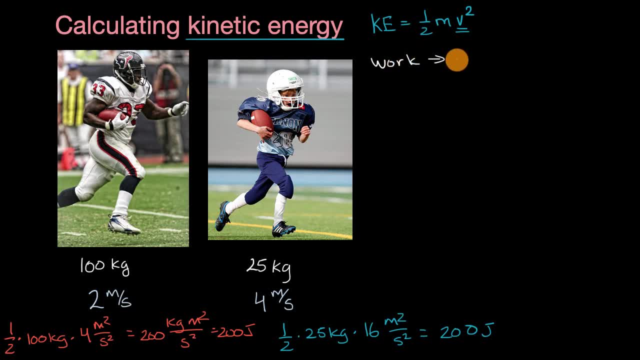 is that you can use work to transfer energy to a system or to an object somehow, and then that energy is that object's capacity to do work again. So let's imagine some object that has a mass m and the magnitude of its velocity or its speed is v. 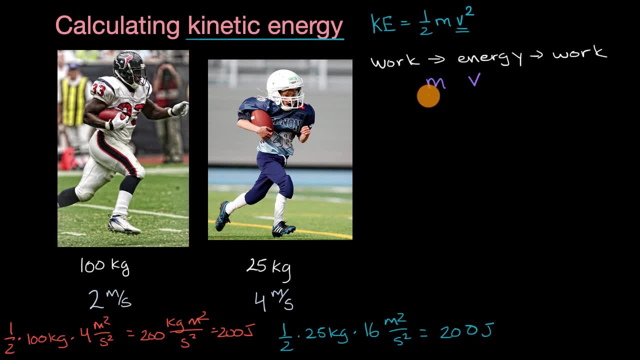 So what would be the work necessary to bring that object that has mass m to a speed of v, assuming it's starting at a standstill? Well, let's think about it a little bit. Work is equal to the magnitude of force in a certain direction. 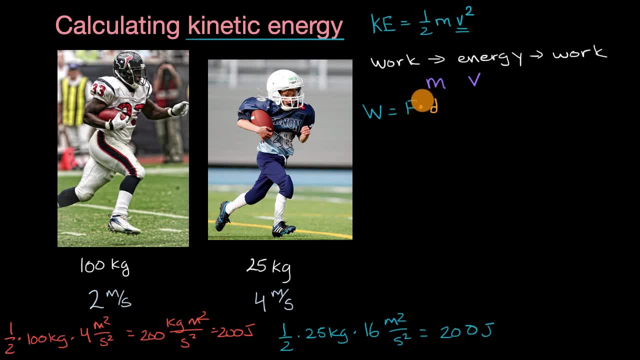 times the magnitude of the displacement in that direction, which we could write like that: Sometimes they use s for the magnitude of displacement as well. And so, what is the force? the same thing, as We know that the force is the same thing as mass times, the acceleration. 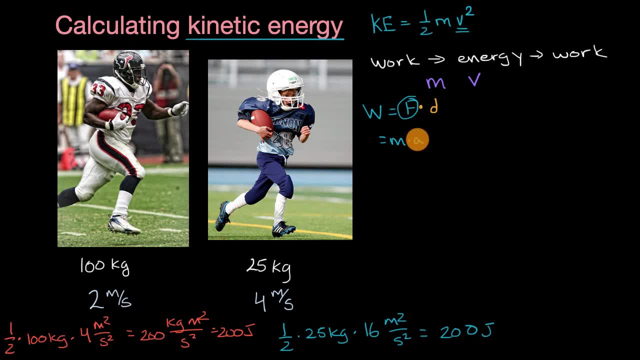 And we're going to assume that we have constant acceleration. just so that we can simplify, We're going to use our derivation here. And then what's the distance that we're going to travel? Well, the distance is going to be the average magnitude of the velocity.